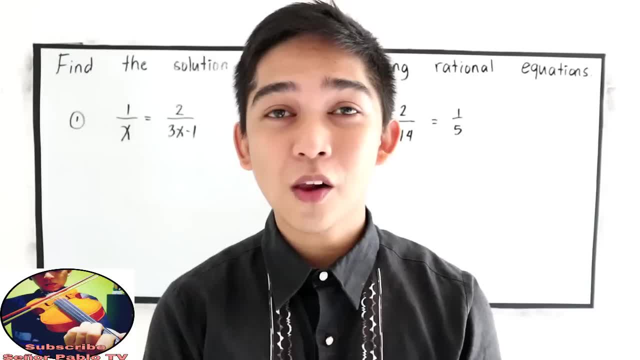 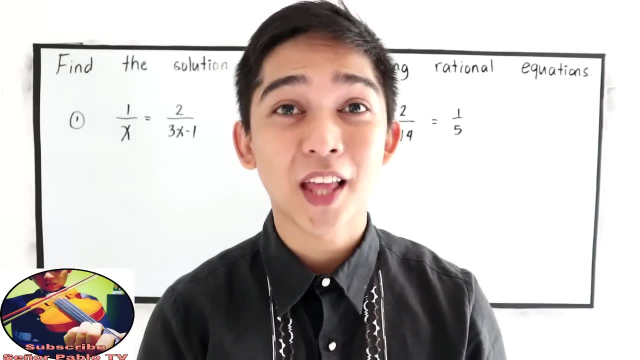 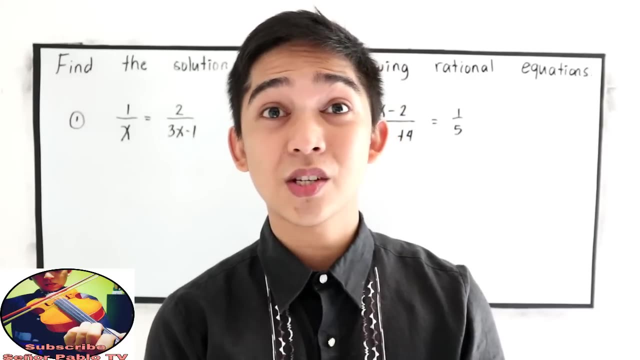 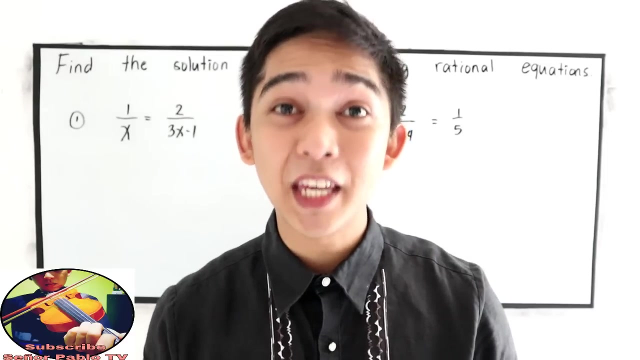 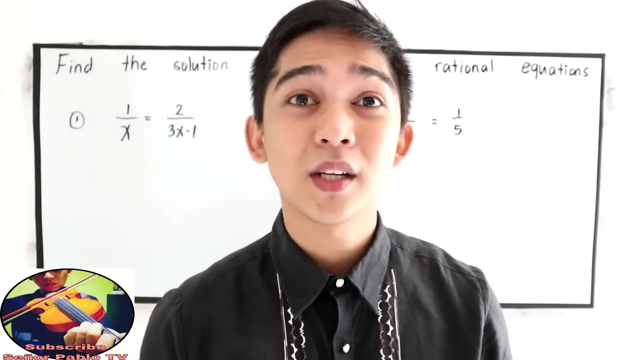 Today we will be discussing solving rational equation, But first let us have a short recall about rational equation. A rational expression is an expression written in the form P over Q, wherein Q must not be equal to 0. Because if Q is equal to 0, that will give us an undefined 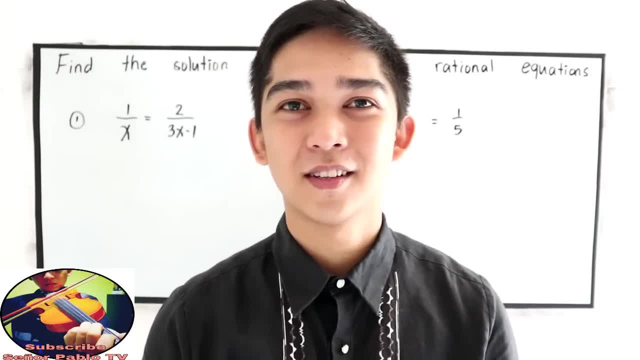 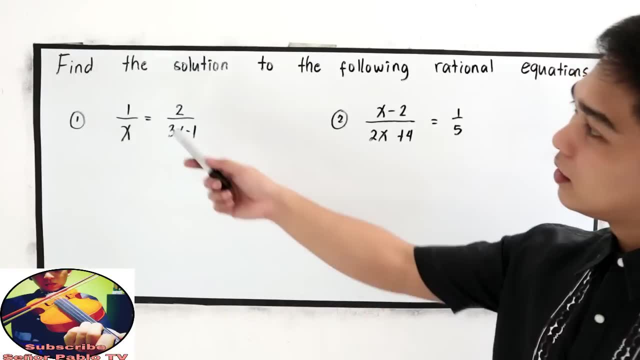 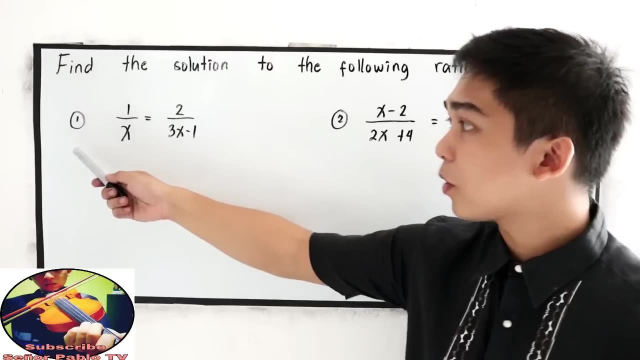 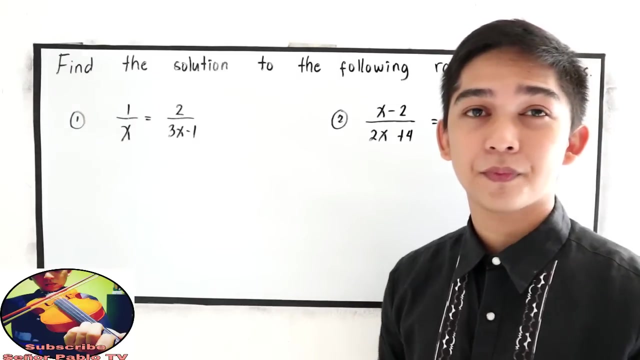 expression That will give us undefined. Now let us try number 1.. Our direction is find the solution to the following rational equations: Number 1, 1 over x is equal to 2 over 3x minus 1.. So we are going to find the value. 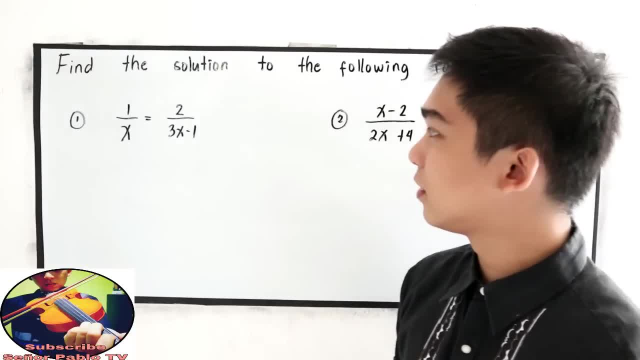 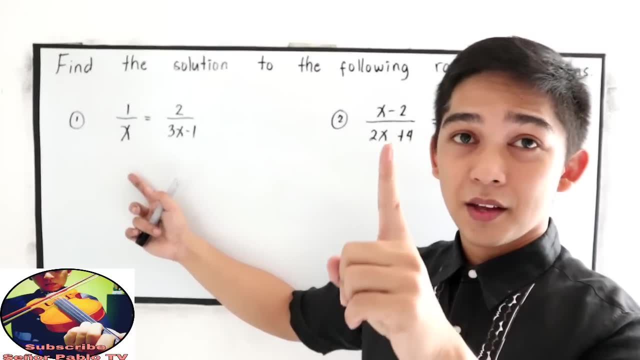 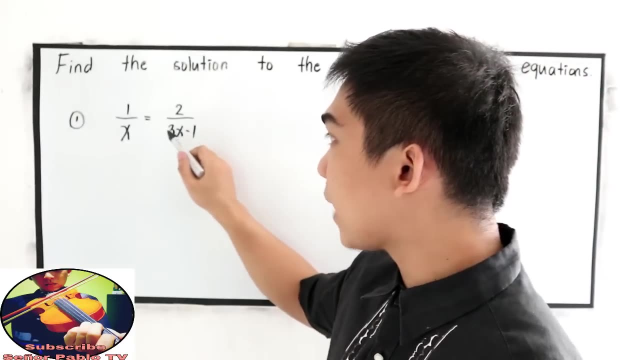 or values for x. So there are two possible ways to solve this equation. The easiest one is using the cross multiplication. So to cross multiply 3x minus 1 is equal to 2 over 3x minus 1.. So we are going to find the values for x. So there are two possible ways to solve. 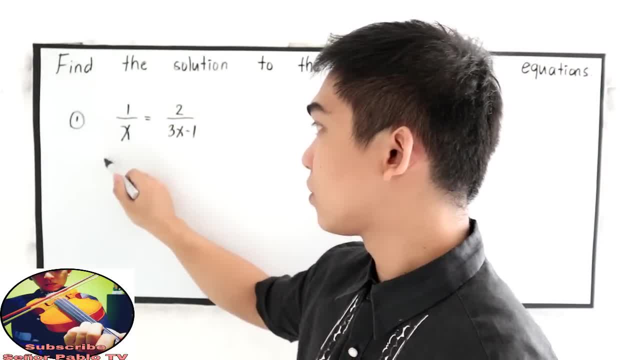 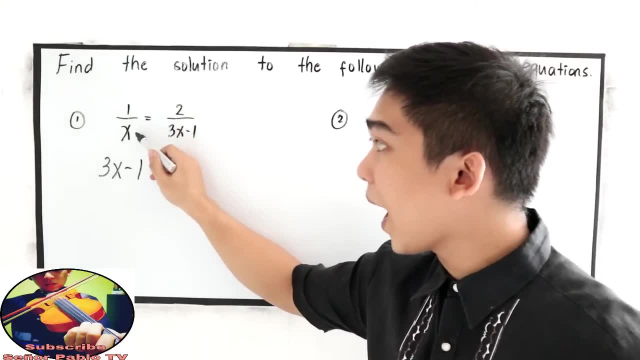 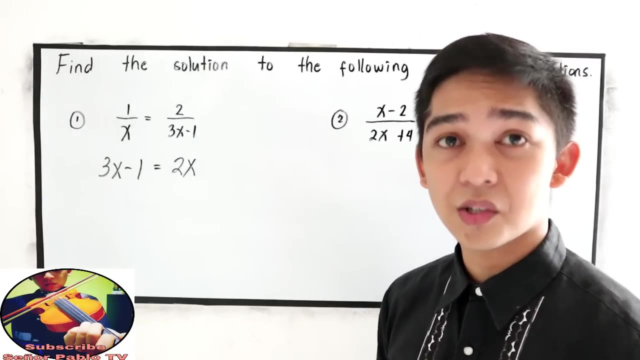 this equation, Number 1, 1 over x is equal to 2 over 3x minus 1.. So that is 3x minus 1.. Copy the equal sign, Then x times 2.. That is 2x. Now combine like terms, Sorry, So 3x. 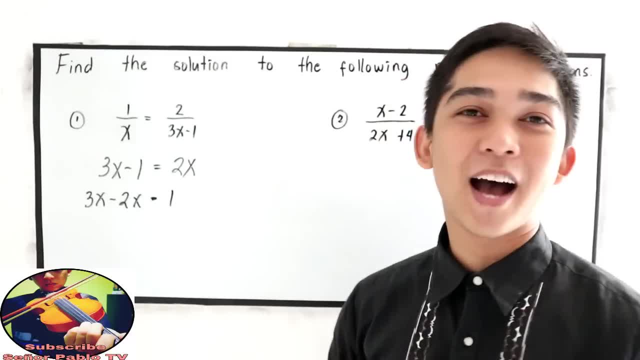 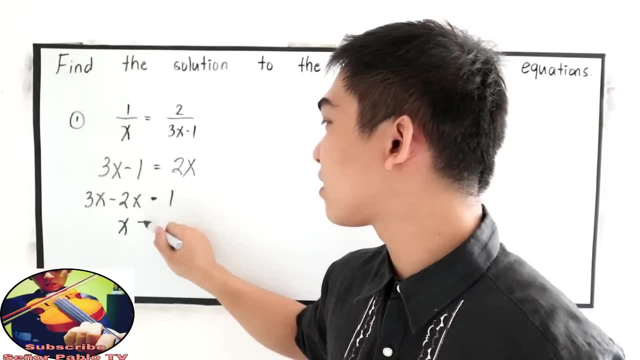 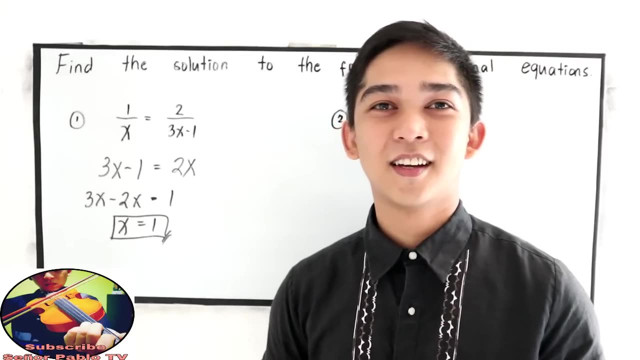 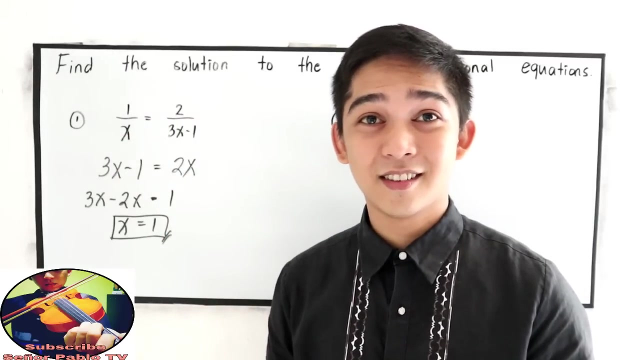 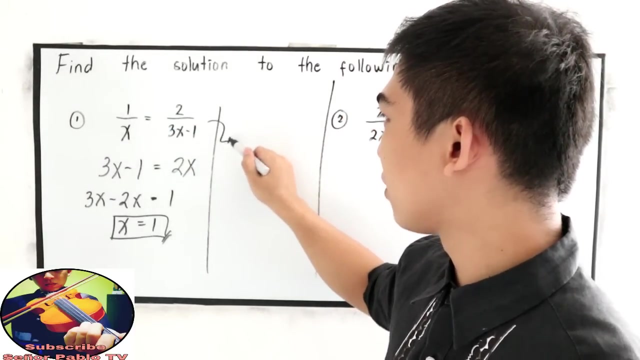 minus 2x is equal to positive 1.. Next, 3x minus 2x, that is x, is equal to 1.. Okay. The other way is using the or getting the LCD. Let's say okay. the other way is- I will write my solution here: 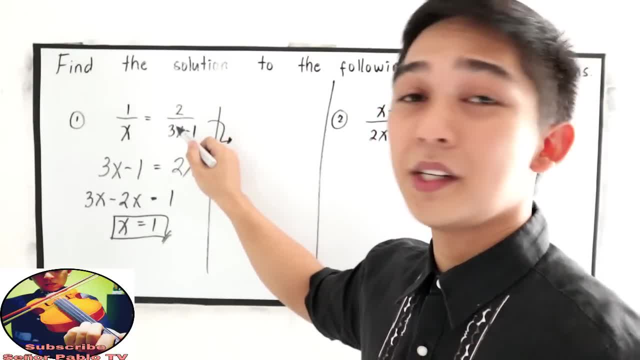 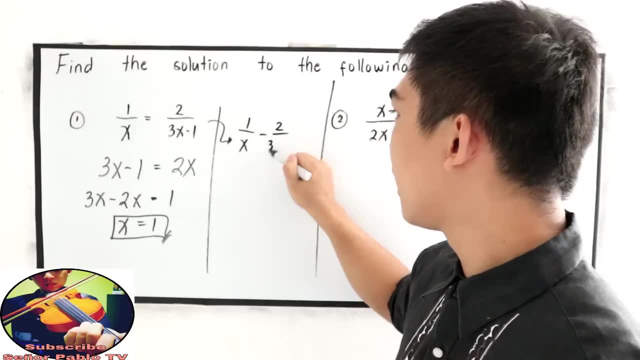 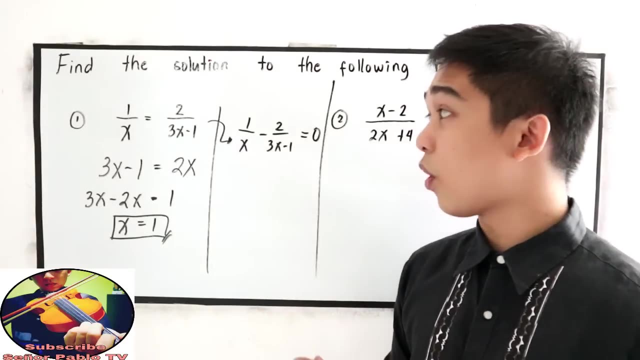 So I'm going to transpose 2 over 3x minus 1.. So that will become 1 over x minus 2 over 3x minus 1 is equal to 0.. We transpose 2 over 3x minus 1.. 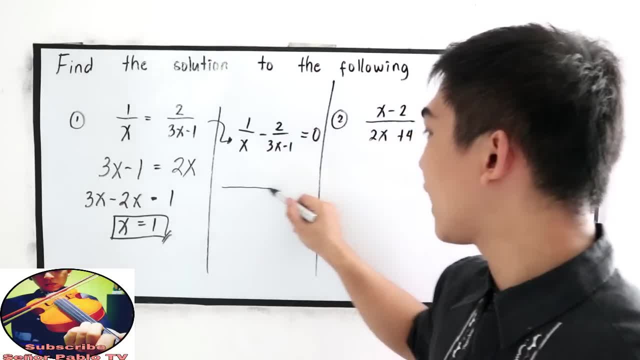 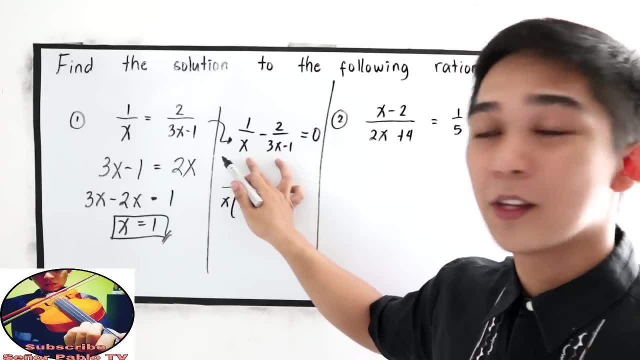 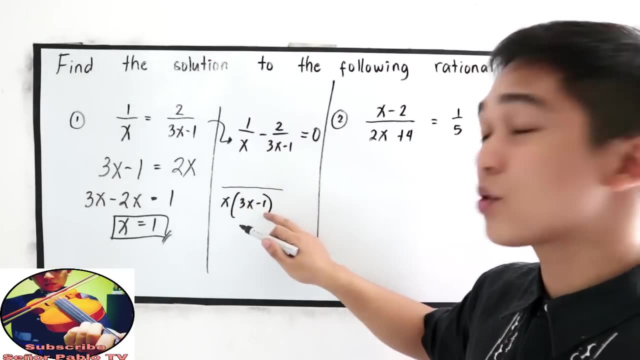 Now find the LCD. Our LCD is x times 3x minus 1.. Our denominator So x times 3x minus 1. divided by x, that is 3x minus 1 times 1, 3x minus 1.. 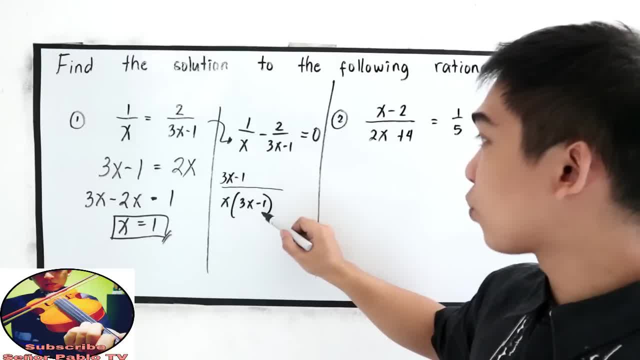 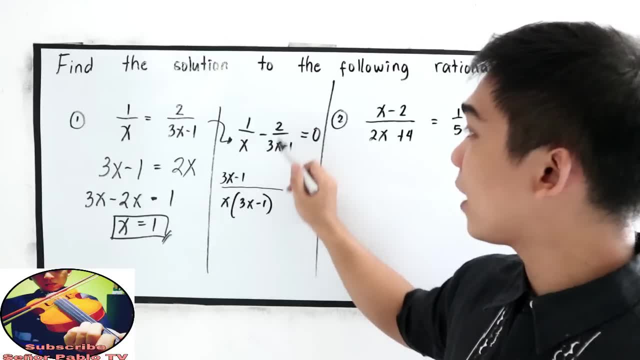 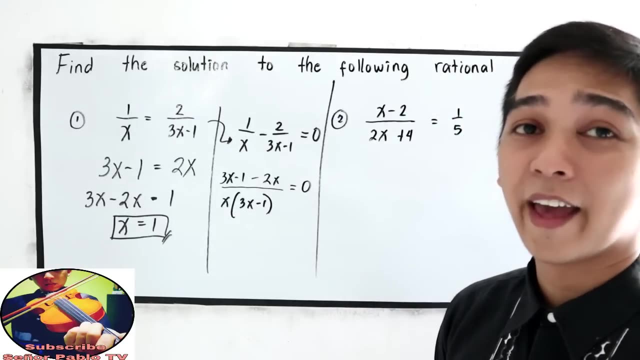 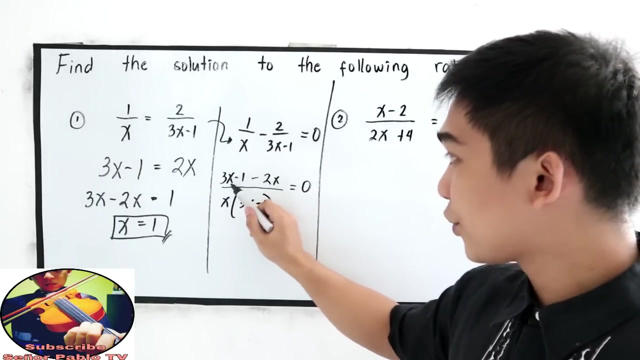 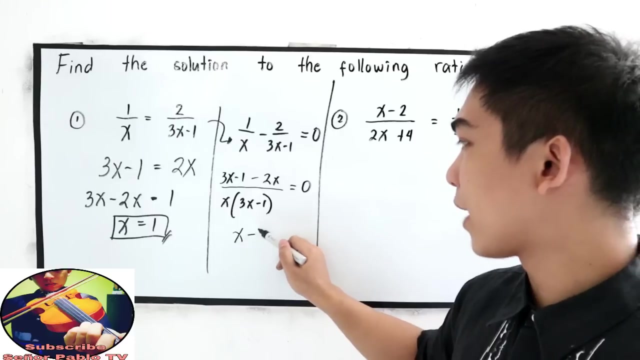 Next: x times 3x minus 1 divided by 3x minus 1, that is x multiplied by 2 negative 2x is equal to 0.. And next combine like terms in our numerator: 3x minus 2x, that is x. then copy: minus 1 over x times 3x minus 1 is equal to 0. 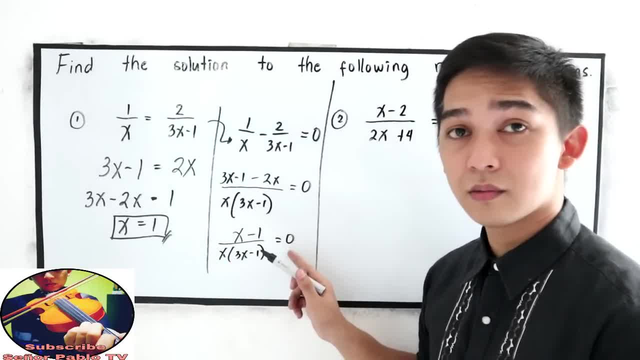 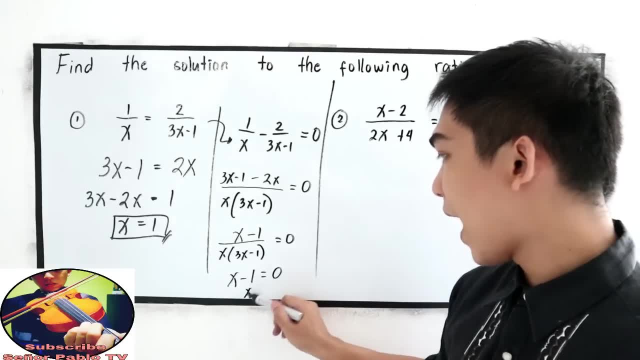 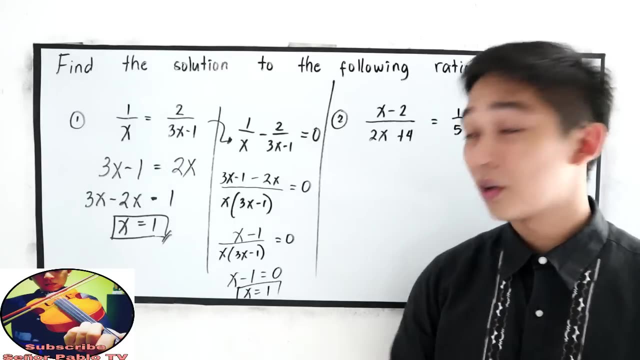 Now our denominator multiplied to 0,, that is to become 0. So next will be: x minus 1 is equal to 0. And now x is equal to positive 1, which is the same. So you will choose which method you're going to use. 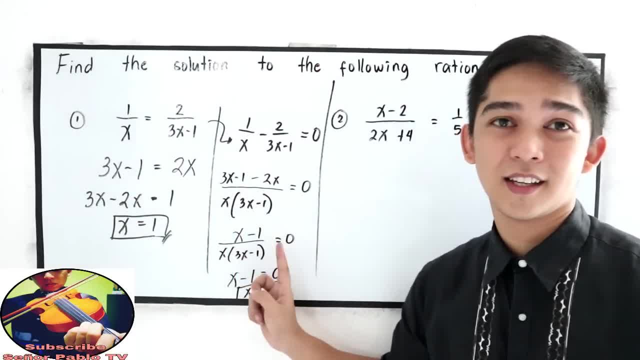 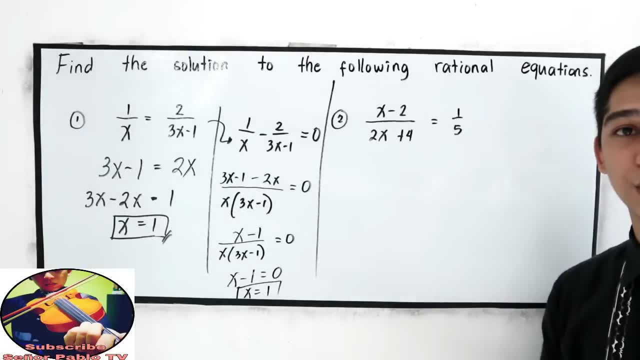 You can use the easier one or the moderate one. Now I want you to try number 2.. x minus 2, all over 2x plus 4.. This is equal to 1 over 5.. If you want to try, you can pause the video. 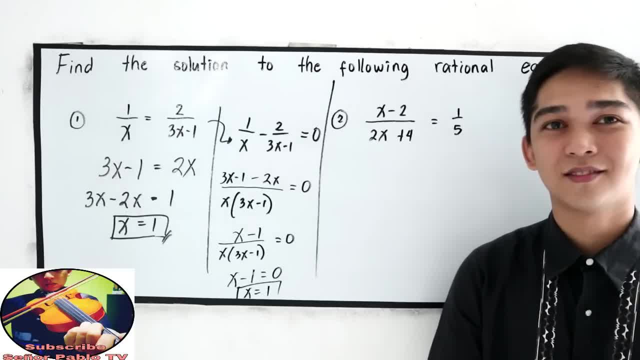 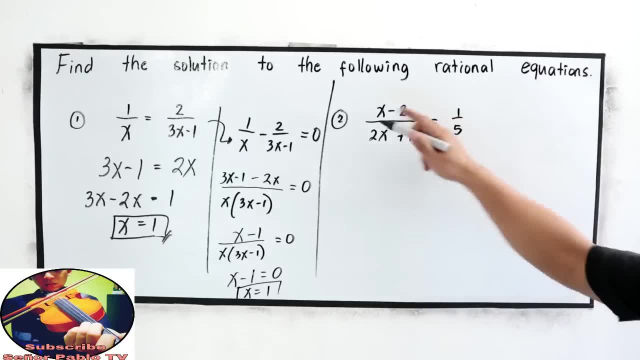 And, after answering, resume watching. Okay, that's right, Let's use the easiest way: Cross multiply. That will become 5 times x minus 2.. Next, 2x plus 4 times 1. Now it will become 2x plus 4.. 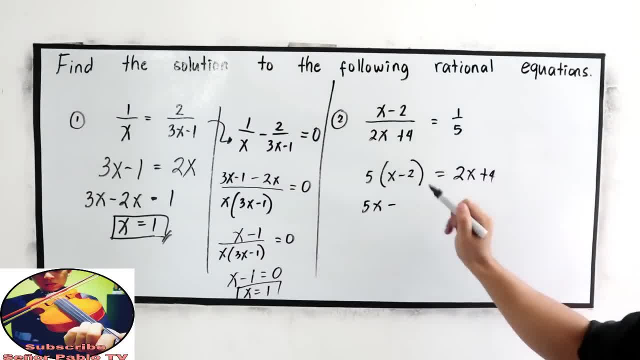 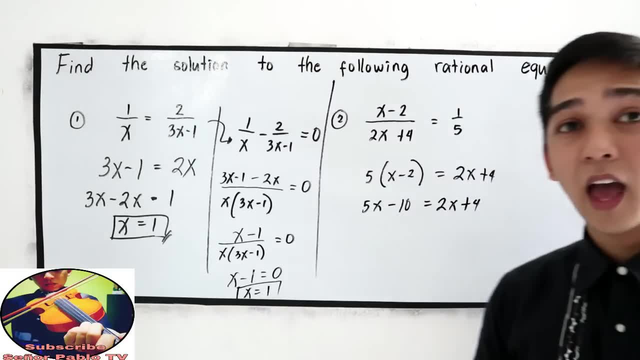 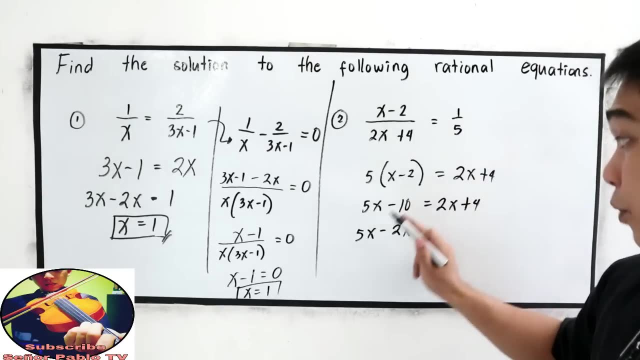 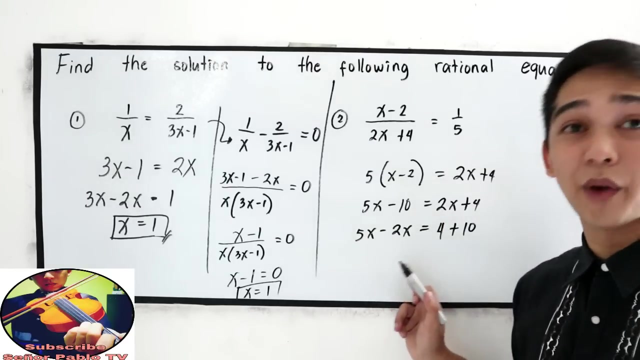 Distribute: 5x minus 10 is equal to 2x plus 1.. And now combine like terms: 5x minus 2x. we transpose 2, is equal to 4 plus 10.. 5x minus 2x.